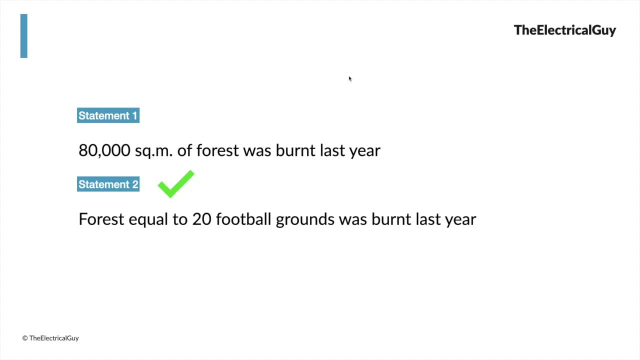 to the size of a football ground. We can imagine the size of a football ground, right, And that is the reason why we could relate to the second statement immediately. Imagining 8,000 square meter ground is tough, But the moment I say 20 football grounds, I have the idea of the size of. 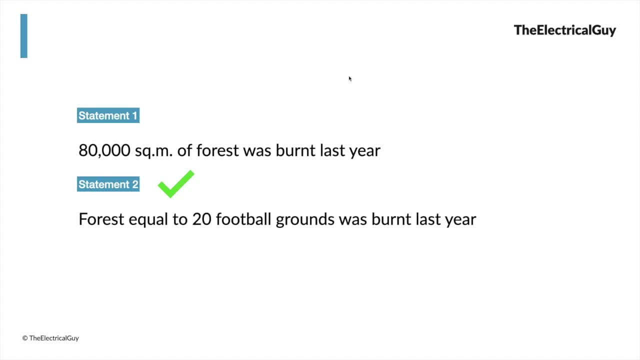 that forest. Well, the bottom line is, we always get a better idea of something if we compare it with something similar. right, And the same thing is also followed in electrical engineering, And it is called the per unit system. We are going to talk about the per unit system for electrical engineers in this video, So 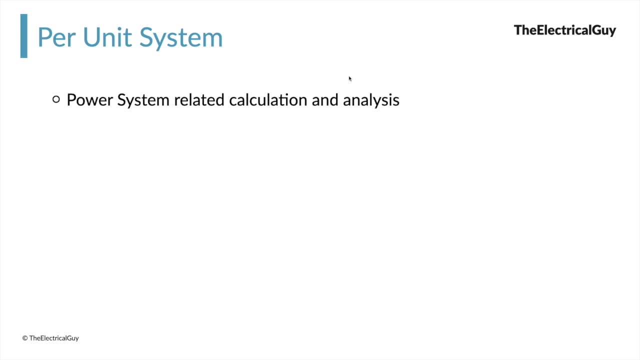 per unit system is generally used in the power system calculations or analysis. It is generally used to calculate short circuit current power flow and machine studies. You will have interaction with the per unit system while studying power system and subjects related to power system. 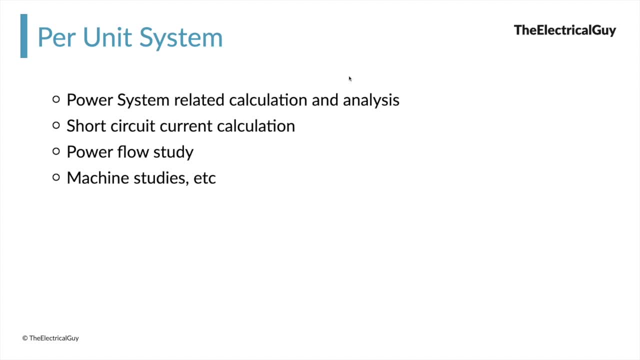 Now, before we understand what is per unit system, let me give you one example. Let's say in a city, average weight of people is 60 kg. Now, using 60 kg as our base value, we can compare weight of any person in the city in terms of the base weight. For example, a person weighing 90 kg would have a per unit weight. of 1.5.. Similarly, if another person is weighing 50 kg, then the per unit weight could be 0.833.. Doing it in this way way makes it really easy to understand. For instance, if a person per unit weight is 1.4,. 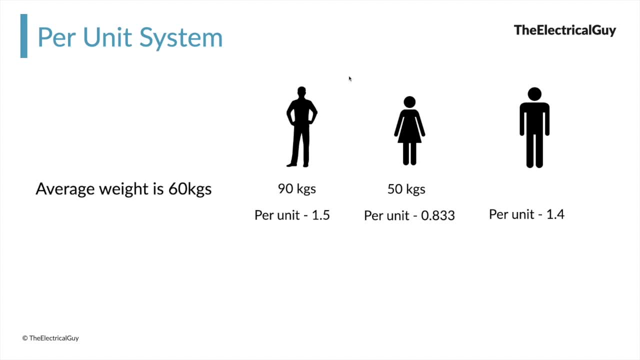 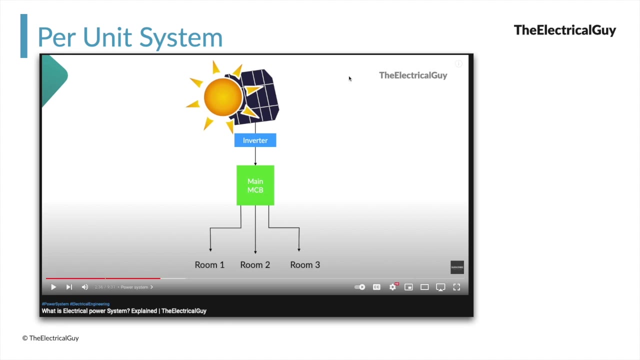 we immediately can identify that this person's weight is more than the average weight, and we can also easily identify its actual weight. To make thing more clear, let me give you example of our power system. By the way, if you want to know what is power system, 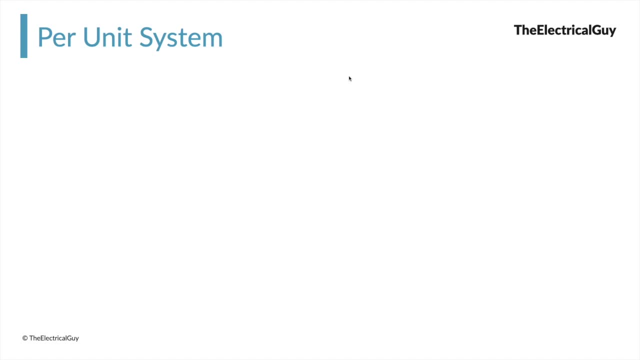 then you can watch my video on that. Link is in the description of this video. We know that we generate electricity at lower voltage, ie 11kV. Then this 11kV is stepped up for a transmission purpose. The voltage range is in between 145kV to 800kV. Then the voltage is 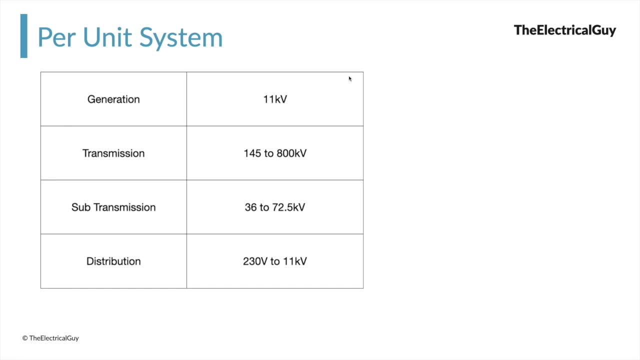 stepped down to a sub-transmission phase in which the voltage level is between 72.5kV to 36kV And further. at the time of distribution, the voltage is further stepped down to 11kV or 440V. 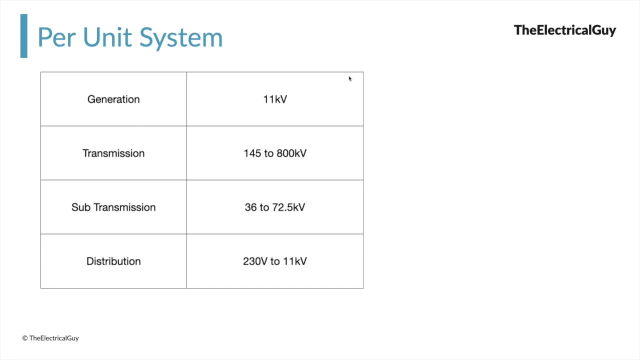 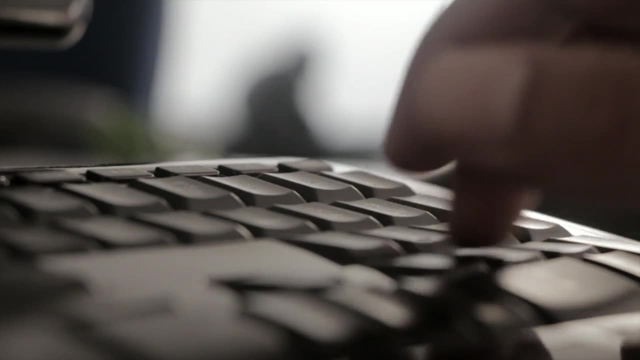 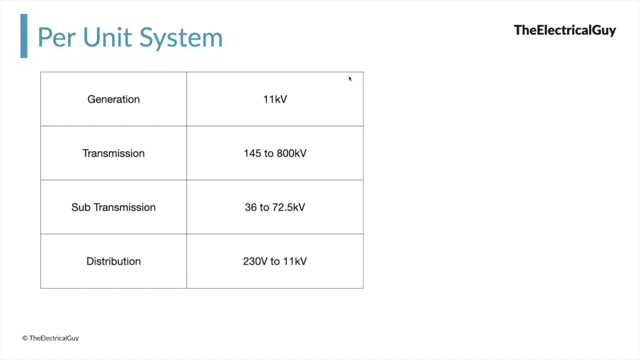 Now imagine you are doing a load flow study for short circuit calculation. You would have to deal with so many different voltage levels which will make the calculation very difficult. So when we deal with the complete power system, where there will be hundreds of generators, 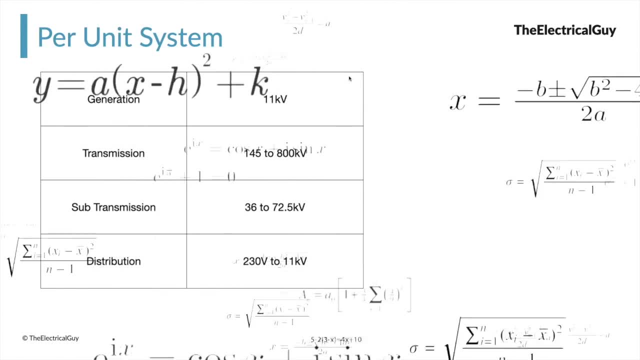 hundreds of transformers, different interconnecting transmission lines. the calculation will definitely get more and more complicated, And per unit system is the solution for this complexity. Just like the weight of the people in the city, we can make a base for the voltage and have much easier calculations. 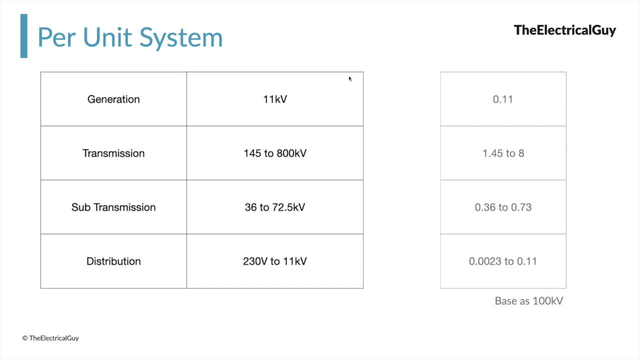 So on the left hand side you can see the voltage values without consideration of per unit system, And on the right hand side you can see the simple values obtained by per unit system method. Here we have considered 100kV as the base value. I will tell you about. 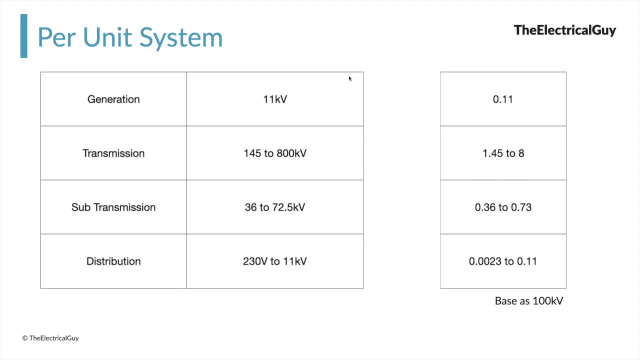 how you can do this in few minutes. You can see here how easy it becomes to identify the values and use it in the calculation. when we use the per unit values, Basically we are dealing with less numbers than earlier, And this is not only applicable for voltages, but also for current power and also for impedance. 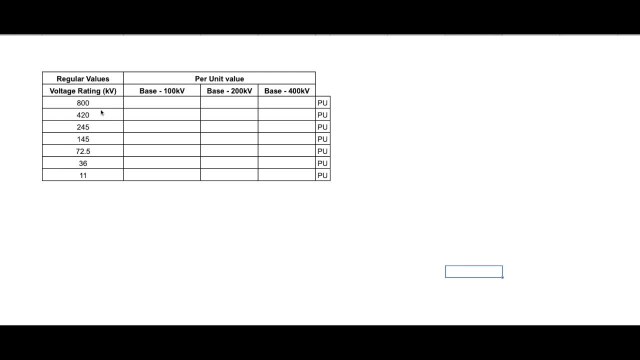 Now we understood why per unit system is important and how it can make the calculation easy. Now let's see how we can get to the next step. How can we get the per unit values? So let us continue with our voltage example, but you can apply the same thing to values. 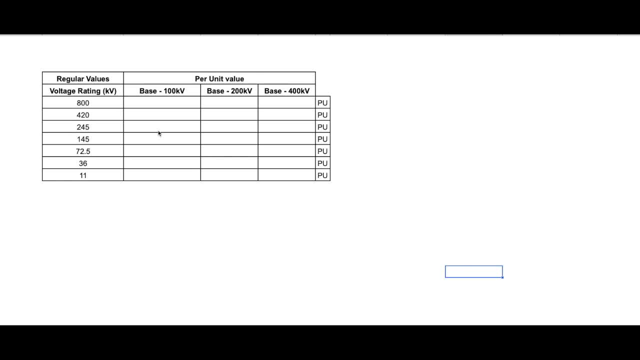 of current or impedance power or any other parameter. So first thing, we need to select a base. Now this base can be arbitrary. Arbitrary means any random value you can select. You can select even 100 kV, You can select 200 kV or even 400kV. 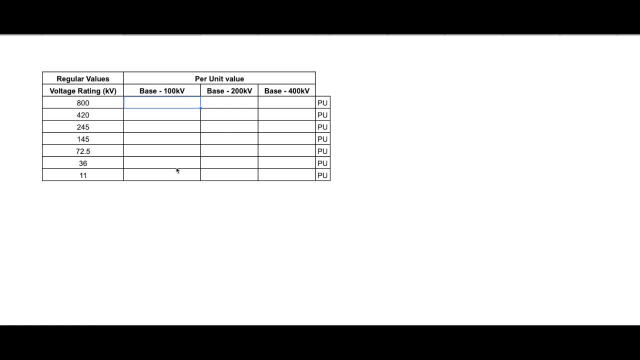 No issues at all. can select any value, any random value. So, first thing, what we will do. let us consider the base as 100 kV. So when the base is 100 kV, what we will do? we will simply divide. 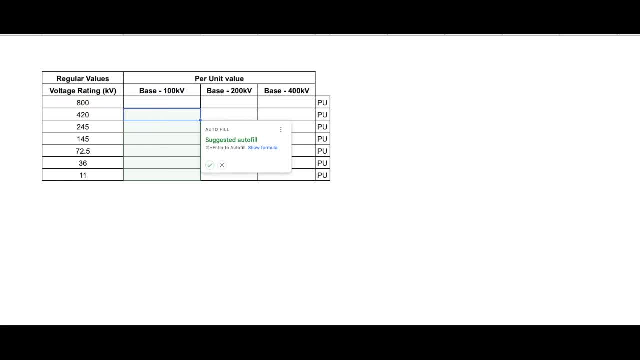 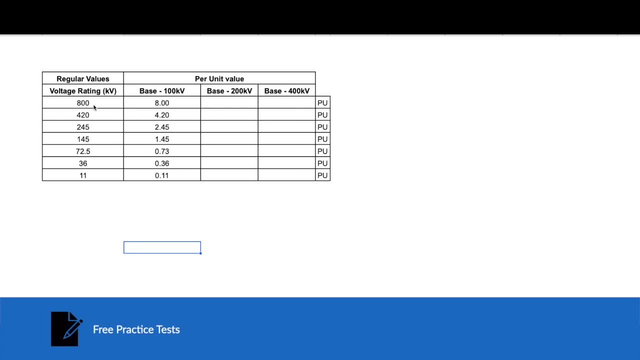 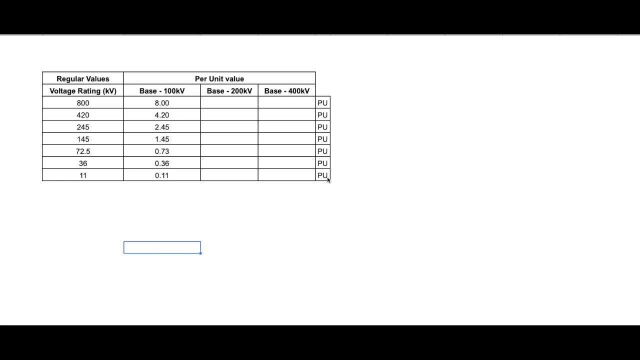 the voltage rating with our base, that is 100.. And we will do the same thing for other voltage rating also. So you see, for 800 kV the per unit value becomes 8 pu. Now, per unit value is always written with the letters pu. that indicates per unit. So similarly you. 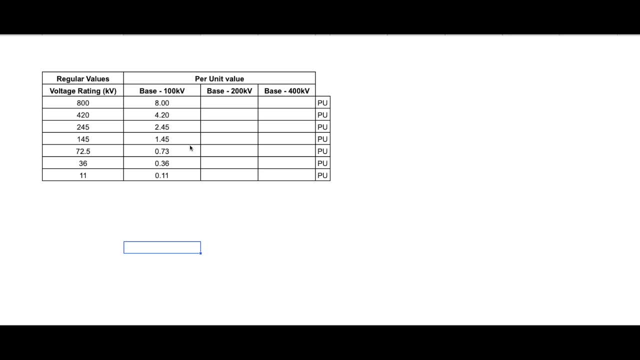 can see, for 145 kV the per unit value becomes 1.45. And anywhere- let us say your power system's base is 100 kV- you refer the number 1.45 and anybody in the power system will understand. okay, this is 145 kV voltage level. So similarly we can also do it considering 200 kV as base. So we will do 100 kV as base. So similarly, we can also do it considering 200 kV as base. So we will do 100 kV as base. So similarly, we can also do it considering 200 kV as base. So we will do. 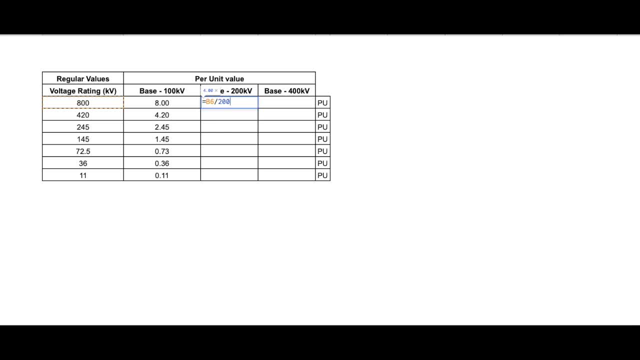 what we will do will divide the voltage rating with our base And you see, you get all the per unit value. Similarly, you can do it considering 400 kV as base. So you can select any base for your calculation and you are good to go. There is no rule as such that you should select. 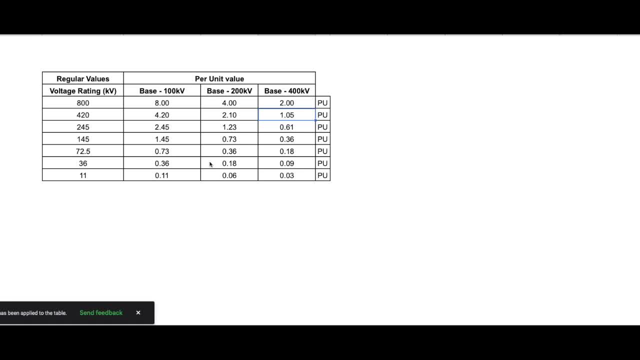 this number or you should select that number. No, it is not like that. Any random value can be selected. Since here we used only one value as our base, it is also called as per unit values with single base. Please note, as I said, whenever per unit values are. 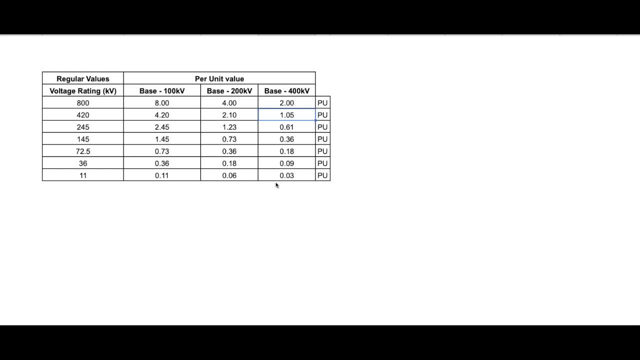 given. they are always pure numbers and always written with PU, which stands for per unit. In this way, calculations are simplified because quantities expressed as per unit do not change with when they are referred from one side of the transformer to the other. This can be a huge advantage in power system analysis where large number of transformers are connected. 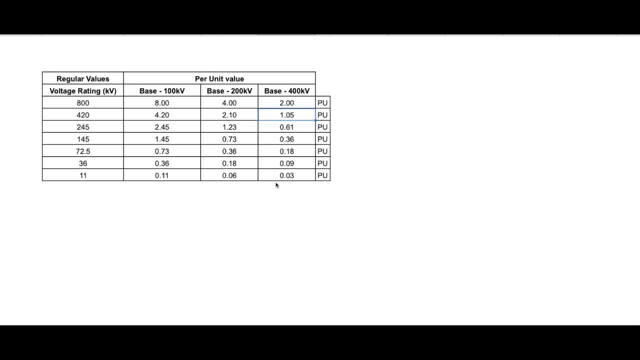 And this method can also be used for impedance, short circuit, current power, etc. The main idea of a per unit system is to absorb the large differences in absolute value into base relationship. Thus the representation of element in the system with per unit value becomes more uniform. 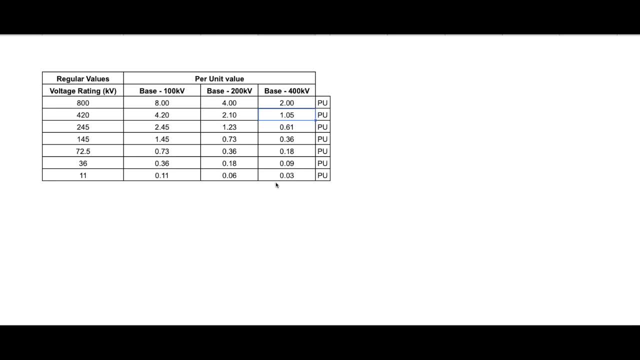 So also, if somebody is referring, let's say, power in per unit system, then you should know the base that has been considered. Without the information of the base it would be difficult to do any calculations. So even if somebody says ki power is 1 PU, Now you do not know. 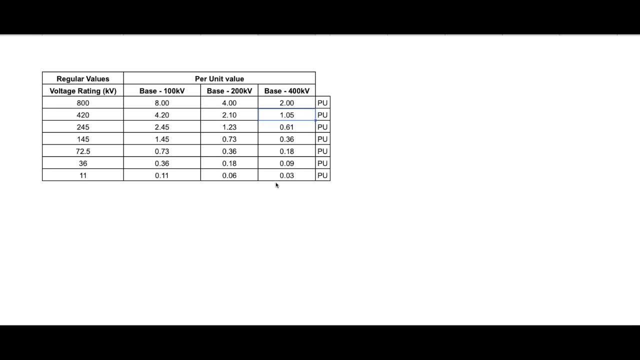 what is the base, so you cannot calculate what could be the actual power. So it is important that you know the base which was considered while getting the per unit values. So this is how per unit system can help you make calculation little easy, and that's. 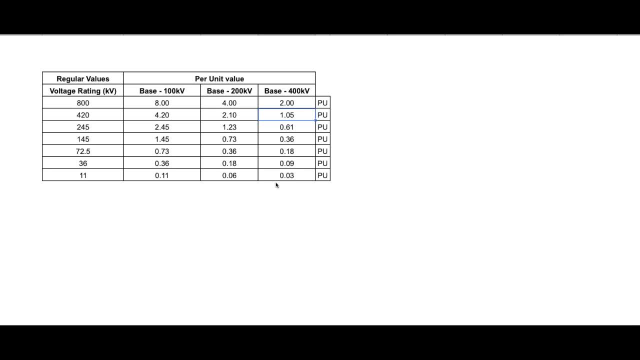 why this system is widely used. Of course, nowadays computer does all the calculation, but the results are still given in the form of per unit system. I hope you found this video helpful and if you did, then please like the video and do share it with your friends. 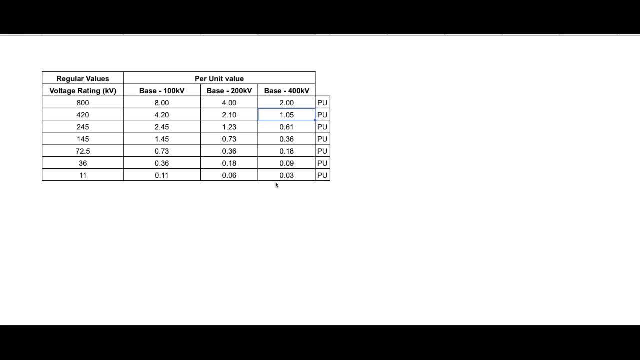 That's all I ask. That's all for this video. I will see you in the next one, Bye, Bye you in my next one, but till then, keep watching, keep learning. 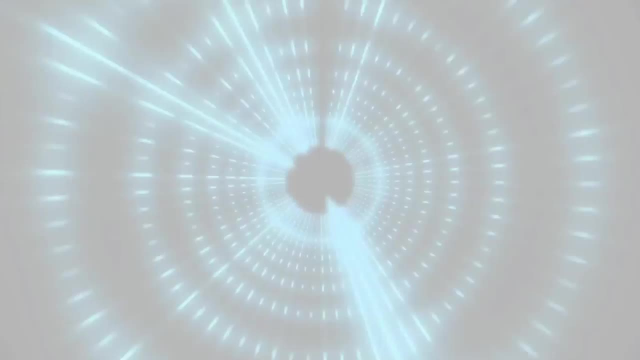 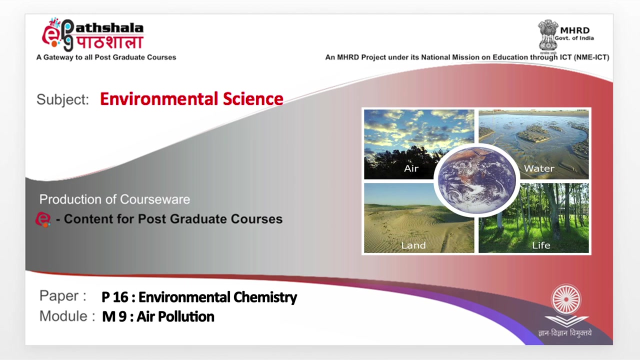 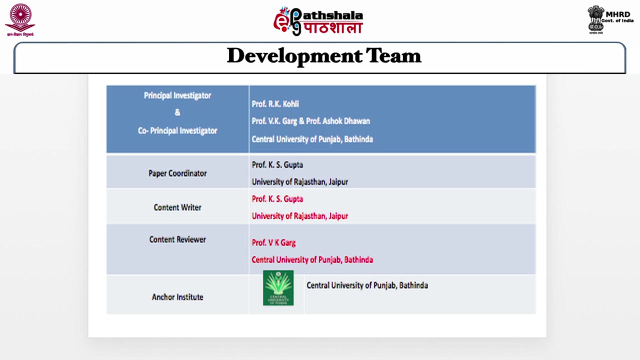 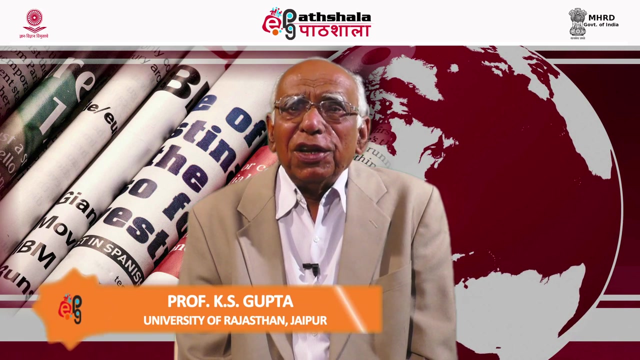 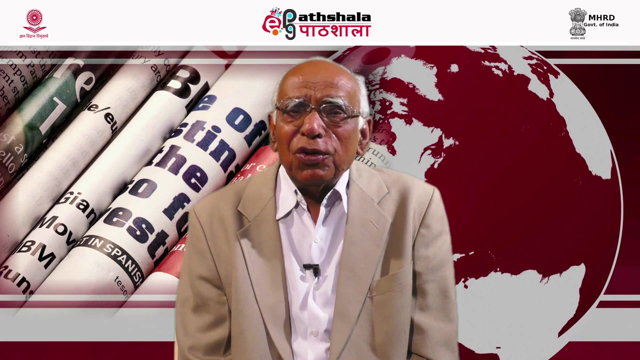 Welcome to EPG Parts Sala. This module will deal with air pollution. The phenomenon of air pollution is well known. Everybody feels it, knows it, but he doesn't mean its scientific meaning. He is also not aware what are real air pollutants, what are their sources and